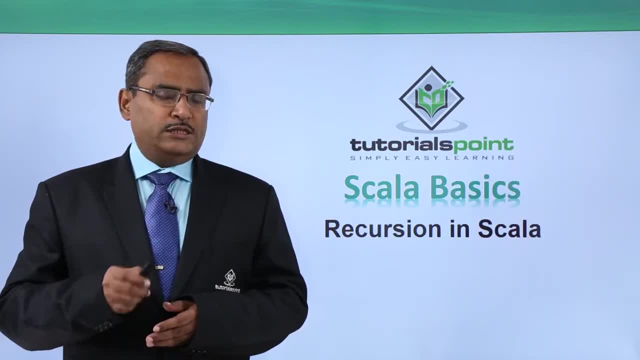 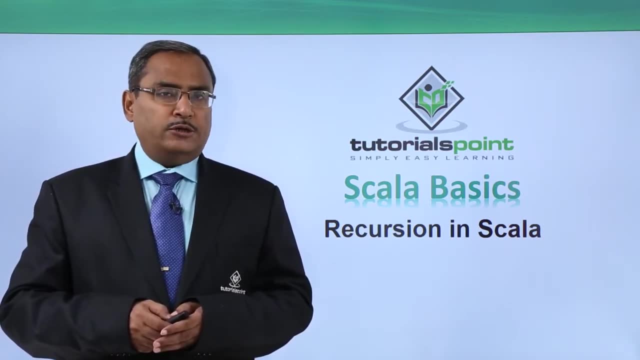 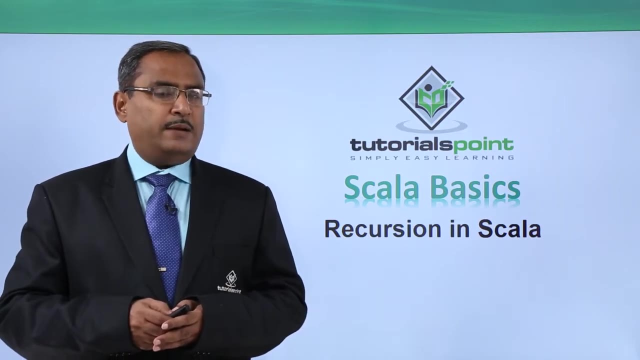 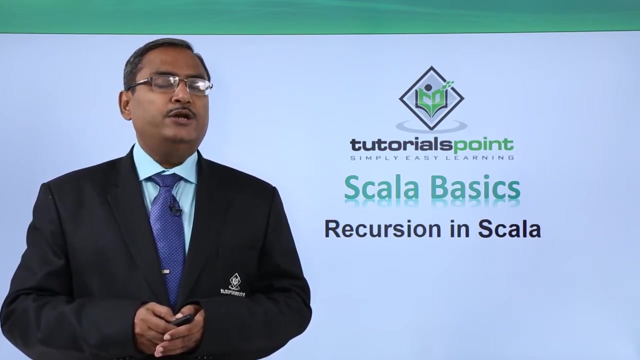 Scala supports recursion, So in this video we'll be discussing recursion in Scala- Recursion. we know that in case of recursive algorithm, the same function will be called from itself, either directly or indirectly, And one recursive function must have some termination logic, also known as the base condition. So let us discuss on this recursion in Scala into more. 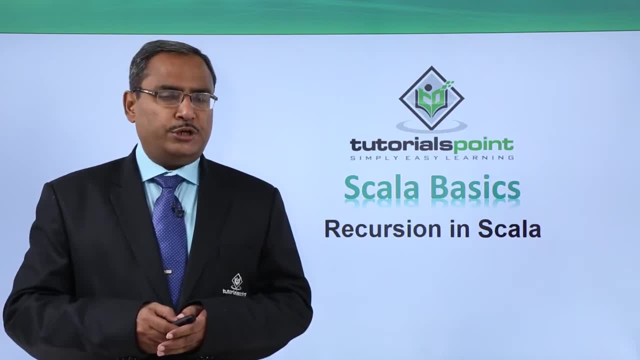 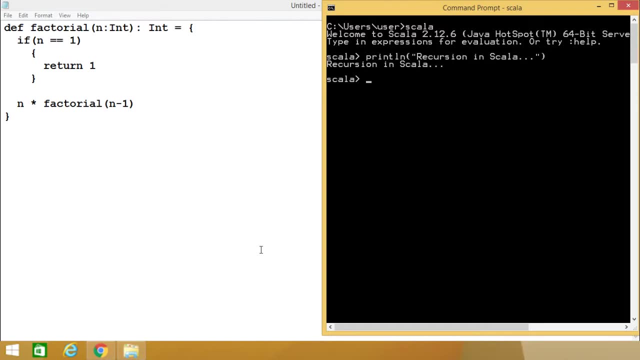 details with one demonstration. So here is the demonstration is following. So in this video we are discussing recursion in Scala and how we can do the recursion using Scala functions. We know that a function involves in recursion when it makes a call to itself And a recursive function. 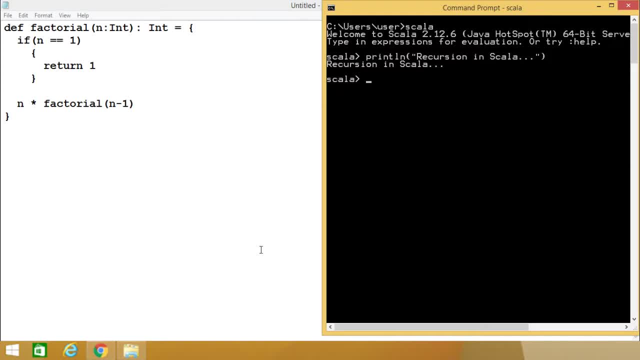 will have two things. two properties are there. Property number one is that for certain inputs the outputs will be known to us, So that is known as the base case for the recursion, And the recursive function will have the function call to itself, either directly or indirectly. 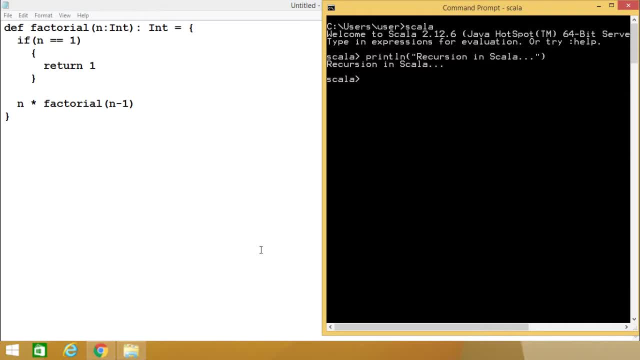 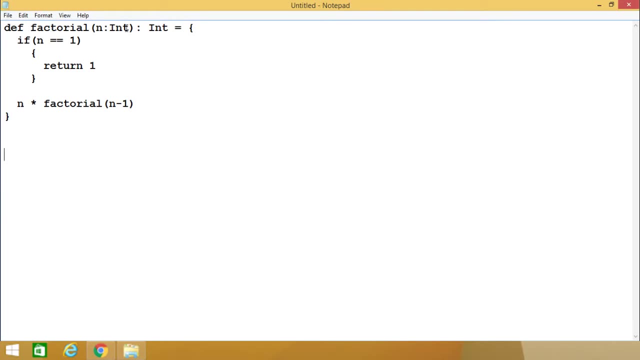 Direct calling means the function calling instruction will be residing within the function body. Indirect calling means it will call another function and that function will in turn call the mother one. So that is known as the indirect recursion. So here we are having one code, So definition, so def. there is a factorial, n is the input argument of the type integer, and 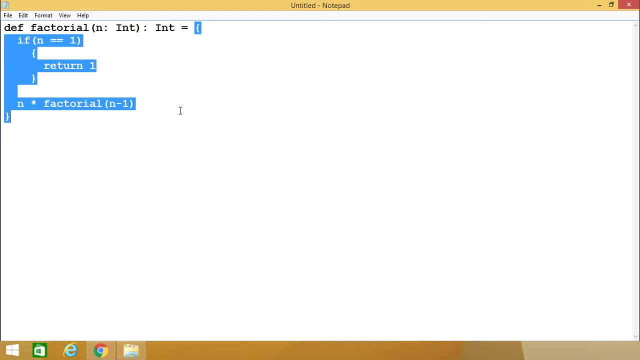 it returns int. And here we are having this body. The function body has been enclosed within curly braces. So if n is equal to is equal to one, then return one. So that means that when the value of n will be one, then the 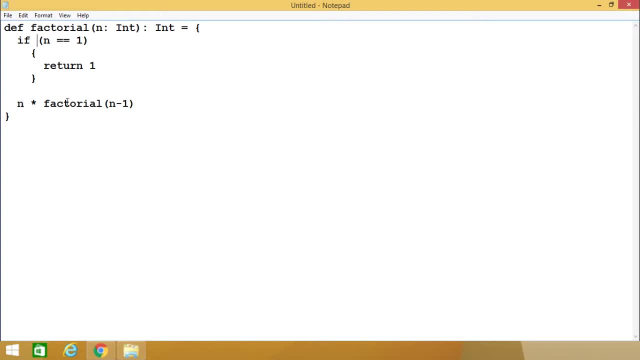 calculated factorial will be also one, Otherwise n into factorial n minus one. So n will be multiplied with the factorial calling the same function, but for n minus one input parameter. So in this way we can do it Here also we can put our OR, so we can also make this one, as n is equal. 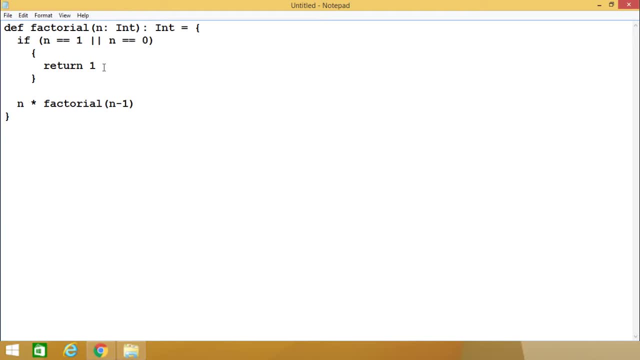 equal to is equal to 0. we know that whenever the value of n is equal to 1 or n is equal to 0, then the factorial value will be 1, so return 1 statement is there, so now let me do a copy of it and let me. 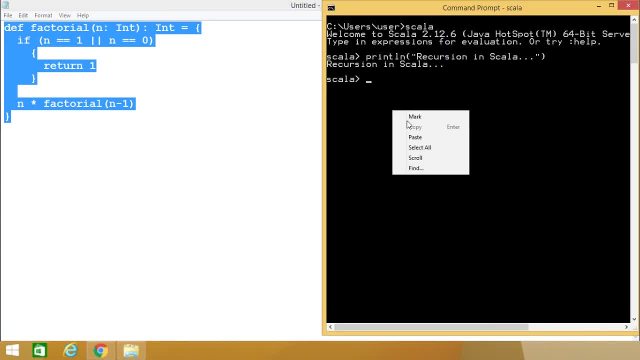 run it in our interactive shell. so i'm going for this best. so now executing the code. so the factorial function has got defined. so now let me invoke it by passing parameter 4, so i'm expecting 24 as output. yes, i'm getting 24. if i pass 5, then i'm expecting 120 will be the output. so in this, 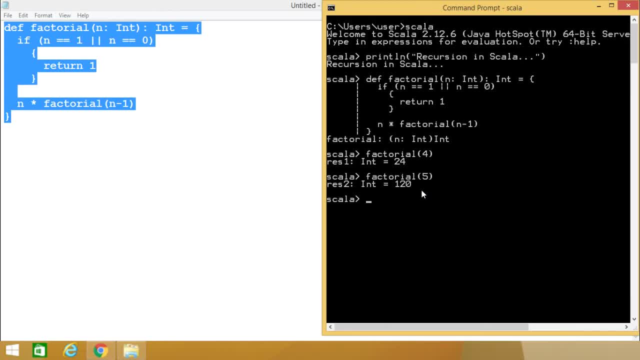 way you can find that, how this particular scalar functions from the scalar functions, how the recursion can be done. that means here we are having one function, that is the factorial. using this factorial we are calculating this particular function, calculating the factorial of the input integer value. here i have passed 4, so its output is 24. here i have passed. 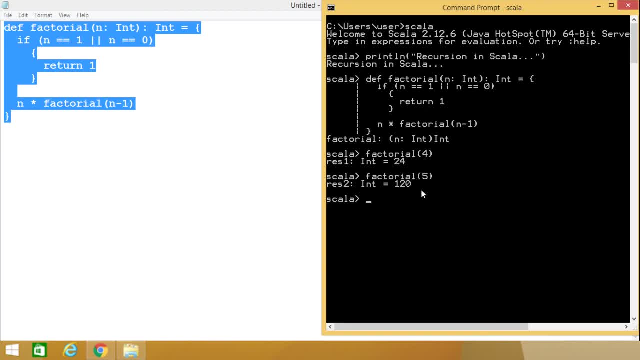 5, so its output is 120. so in this way, how the recursion can get implemented using scalar functions we have demonstrated in this video. thanks for watching this. 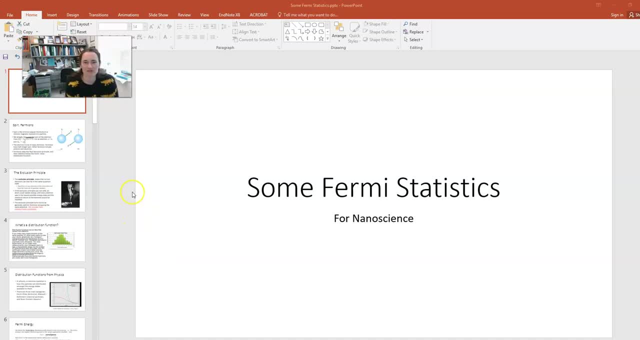 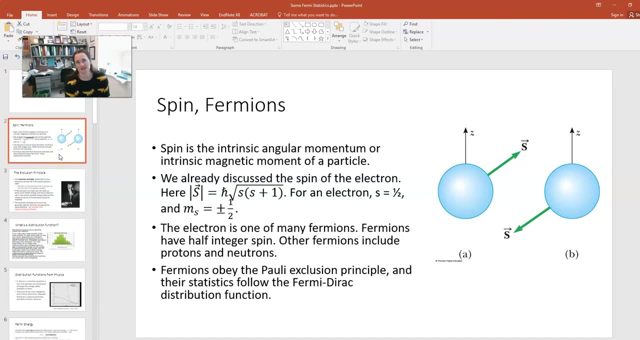 Hi. so today I'd like to talk a little bit about Fermi statistics and fermions and Fermi energies. So to get started with that, let's first remind ourselves of spin. So there's three different main classes of particles in statistical mechanics and those three classes of particles are, you know? 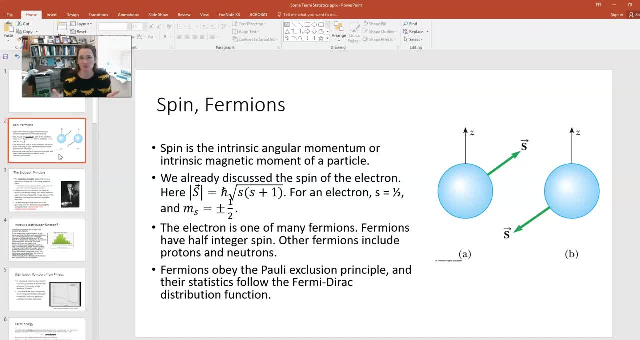 fermions, bosons and then basically classical particles or ideal gas type molecules or particles. And the differences in between these three classes of atoms or molecules, particles, are the spin. So what is spin? Well, spin is the intrinsic angular momentum. 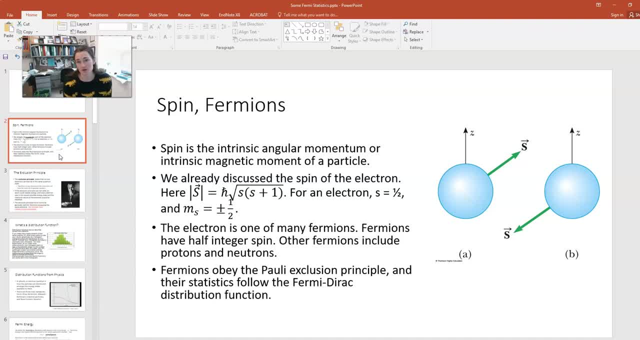 which leads to, of course, an intrinsic magnetic moment of a particle. So lots of people have in their heads this idea of a single particle sitting there and, just like the earth, spins on its axis. it spins right And that would give something an angular momentum. Of course, this idea 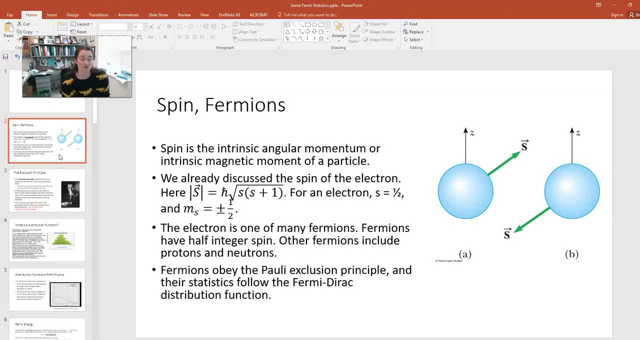 really breaks down. it's not truly valid. For all we know, electrons are point particles. We haven't managed to successfully measure a diameter, for example, so as far as we know, it's infinitesimally small. And so how something that's infinitesimally small spins on its axis? 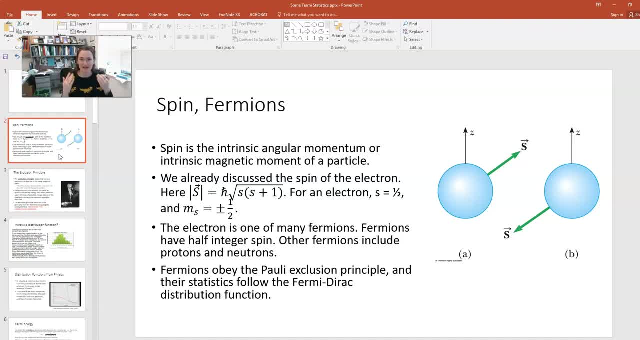 is a really good question. Nevertheless, this idea helps a lot of folks wrap their idea around the fact, wrap their head around the fact that particles do have an intrinsic angular momentum to them. okay, And I think of this these days much like I do in my studies, as think of the